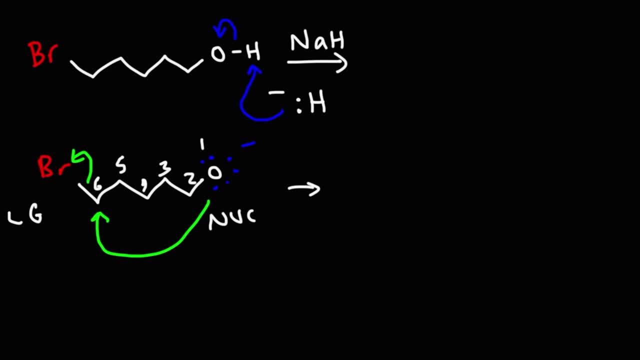 So we're going to get a 6-membered ring. So what we have here is a 6-membered ring, And what we have here is a cyclic ether. Let me draw that better. So that's the answer for this problem. 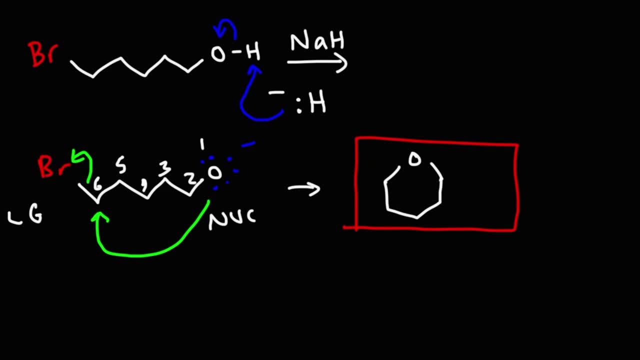 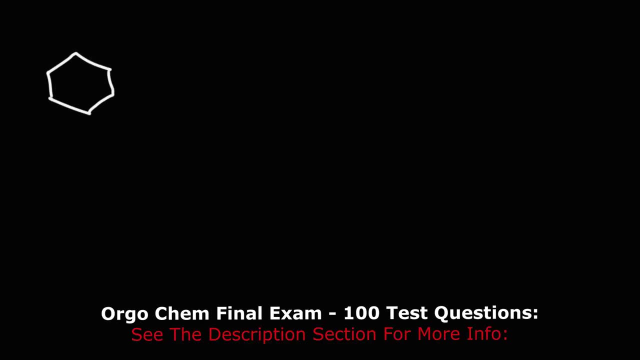 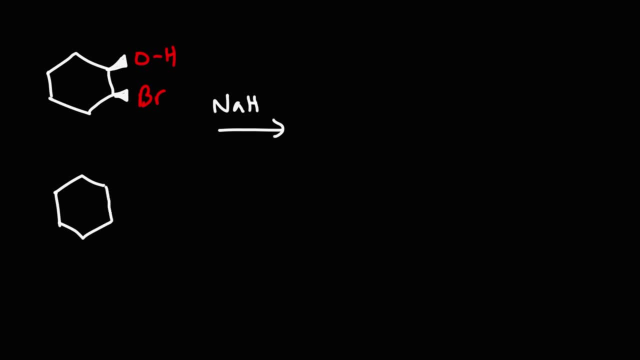 So we're going to react with sodium hydride again. So we're going to react with sodium hydride again. Now, just like before, the hydride ion is going to participate in the acid-base reaction, removing the proton. 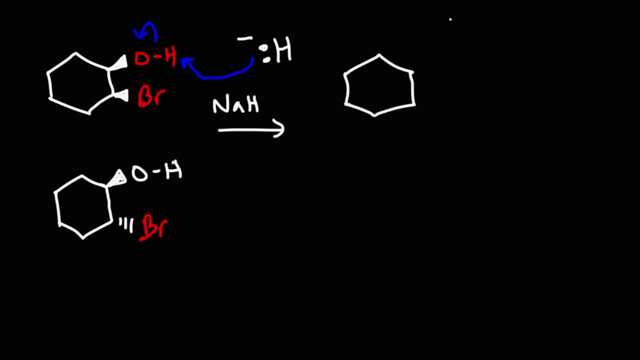 And we're going to get an alkoxide ion And we're going to get an alkoxide ion Which is also part of an alkyl halide. Now, with the other reactant we're going to get the same thing. Hydride can remove a hydrogen. put in the negative charge on that oxygen. 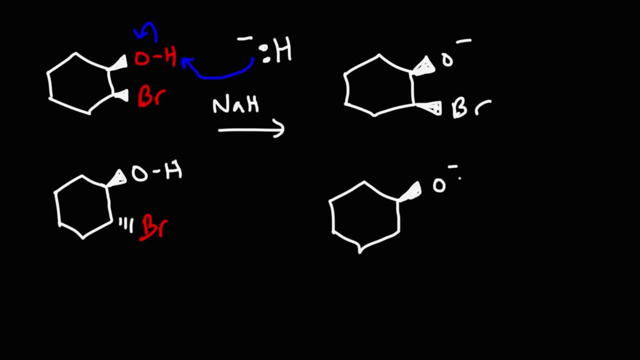 But notice that the stereochemistry is different. But notice that the stereochemistry is different. What do you think is going to happen here? What do you think is going to happen here? Because we have a nucleophile and a leaving group all in the same molecule. 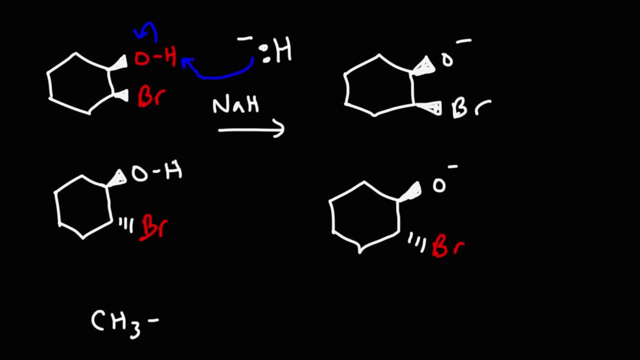 Now, if you recall, in order for the SN2 reaction to work, the nucleophile must approach the substrate from the back. So if bromine is in the front, the nucleophile must be coming in the back. It's not going to come and do a front-side attack. 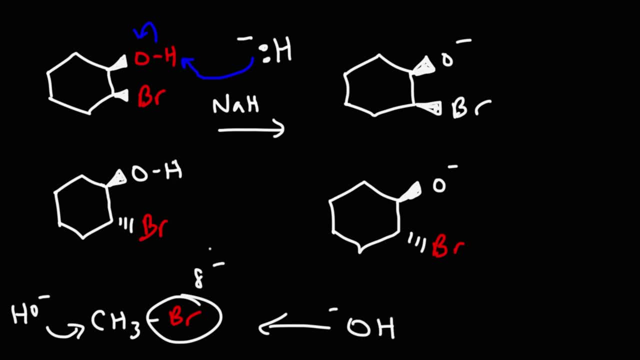 Because hydroxide will be repelled by the partially negatively charged bromine atom. So the front-side attack won't work. Notice that this oxygen and the bromine, they're locked in the same position, They're both in the front. So this negatively charged oxygen, it's not going to attack this carbon. 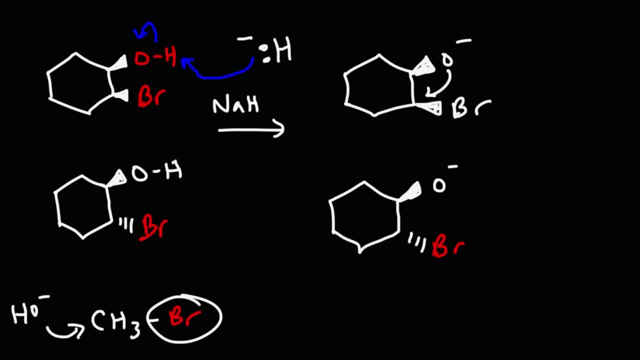 Because in order for it to attack it, it's approaching it from the front. So this is going to stop here. Now for the other one: The bromine's in the back, the oxygen's in the front. So for this one we can get an intramolecular SN2 reaction. 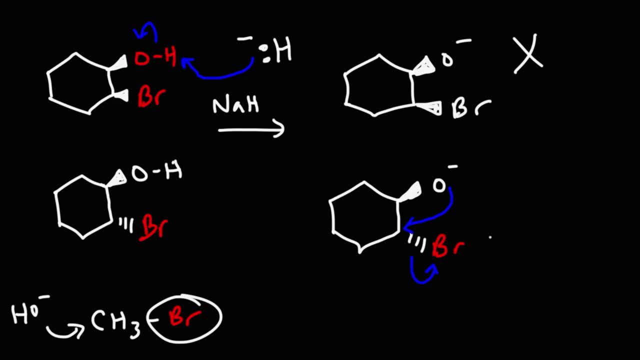 This can attack this carbon, kicking out the Br, And what we're going to get is a special kind of ether. When you get a three-membered ether like this, this is known as an epoxide. But in order to get the epoxide, 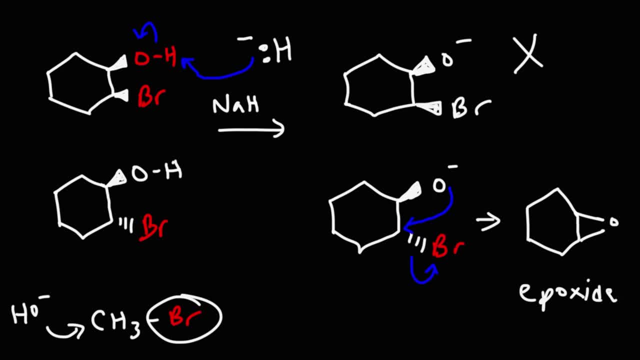 these two groups have to be anti with respect to each other. And then the ether- I mean the epoxide, the carbon-oxygen bonds- will be on the same side, Because this is going to attack from the front, kicking out the Br that's in the back. 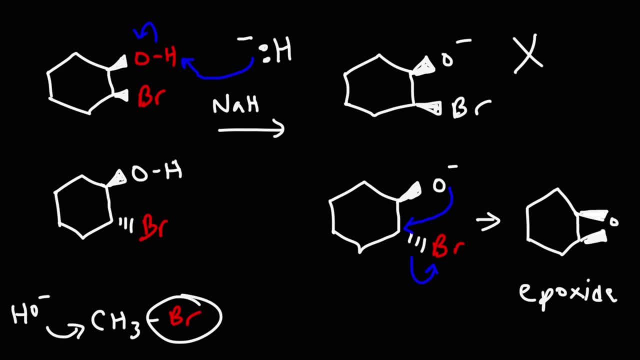 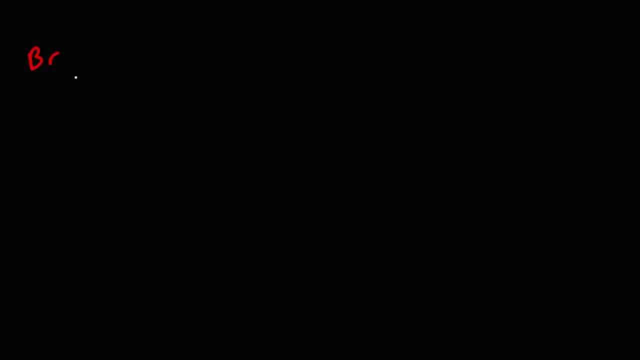 So that's another example of an SN2 intramolecular reaction. Let's look at another example. So here we have 1,5-dibromopentane And we're going to react it with ammonia. Now this particular reaction can give us a mixture of products. 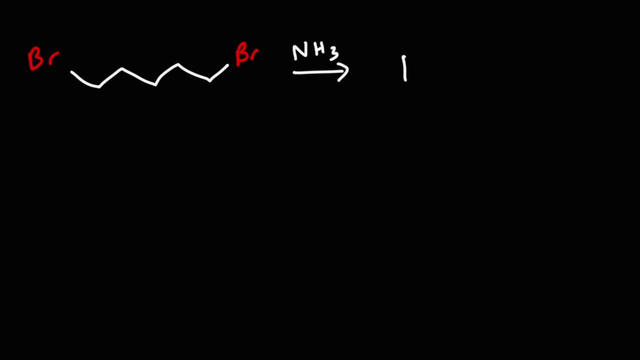 But we're going to focus on the formation of one product, And what we need to do is we're going to propose a mechanism For the formation of this particular product, Even though we can get a lot of other products for this reaction. So feel free to pause the video. 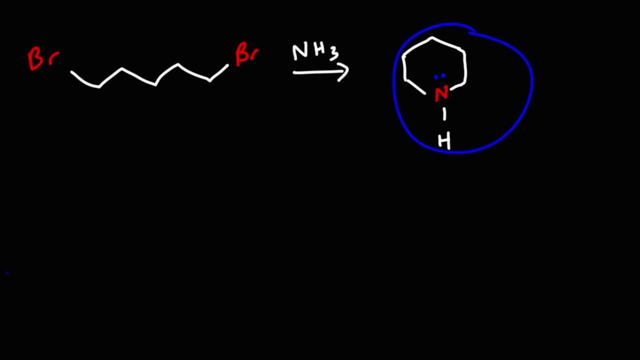 and propose a mechanism for the formation of this product. So ammonia is a nucleophile. It's also a weak base And what we have here is a primary alkyl halide. So we're going to get an SN2 reaction. The nucleophile is going to attack from the back. 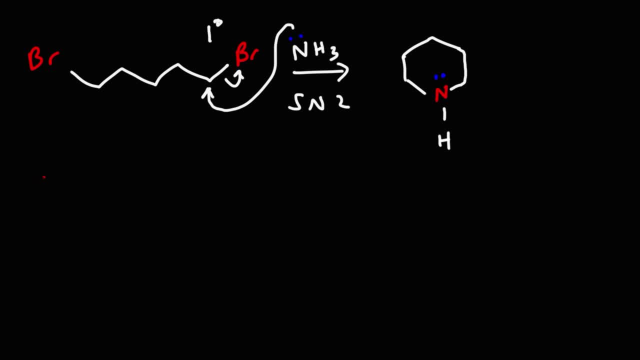 kicking out the leaving Br, So we're going to get this. So right now the nitrogen has three hydrogen atoms attached to it, So it's going to have a positive formal charge because it has a total of four bonds. Now we need this nitrogen to behave as a nucleophile. 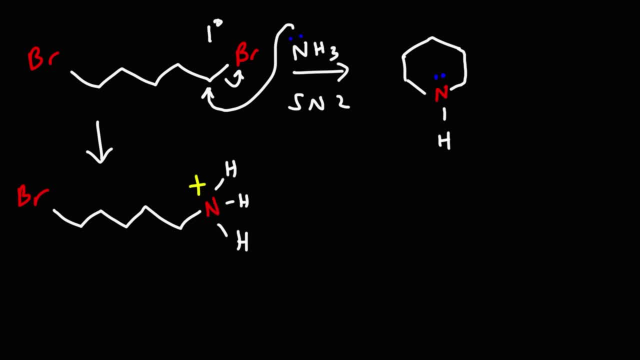 and attack this carbon so that we can close and form the ring. Before we can do that, though, we need to remove a hydrogen from this nitrogen, And we could use another ammonia molecule to do that, So now this NH2 is once again nucleophilic. 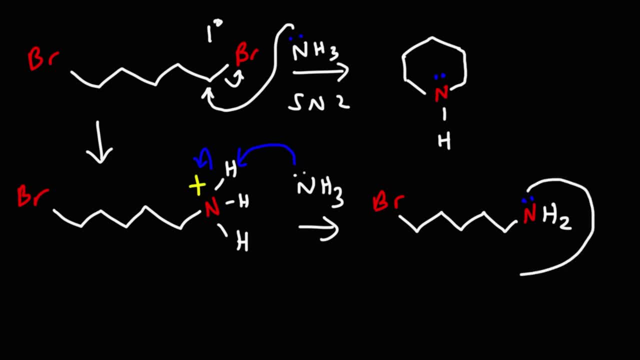 So at this point an intramolecular reaction is going to happen. This nitrogen will attack the carbon, kick out the leaving group. So we can call this number one, two, three, four, five and six. So we're going to get a six membered ring with nitrogen being part of that ring. 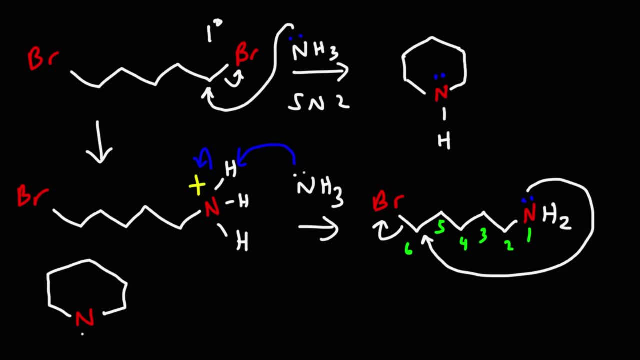 But right now, nitrogen has two hydrogen atoms attached to it And it has a positive. It has a positive formal charge, So we need to use another ammonia molecule to remove this hydrogen. I can definitely draw that better, And this is going to give us our final product, which is acyclic amine. 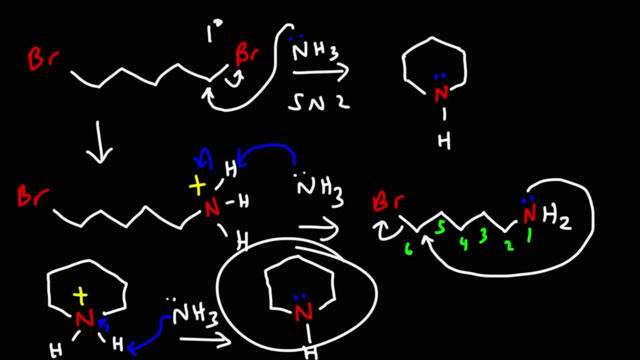 So that's how we can get this product from this particular alkyl halide. Now, keep in mind there's a lot of other products that we can get for that reaction. This is just one of the many products that we can get.